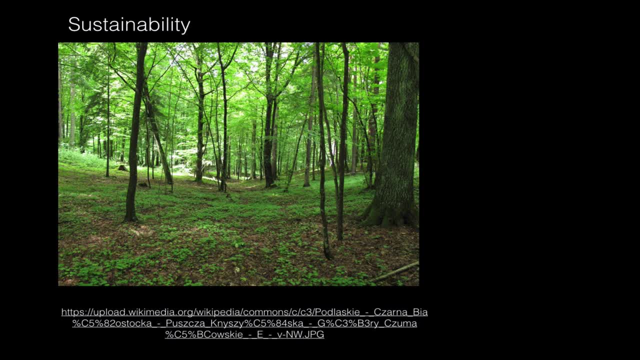 manage it sustainably, or we can manage it unsustainably. So if we're using it sustainably, what this means is we're going to only cut down a certain amount of trees and use them for our benefit, And that's the idea of natural income: That we can use the environment and we can use the goods. 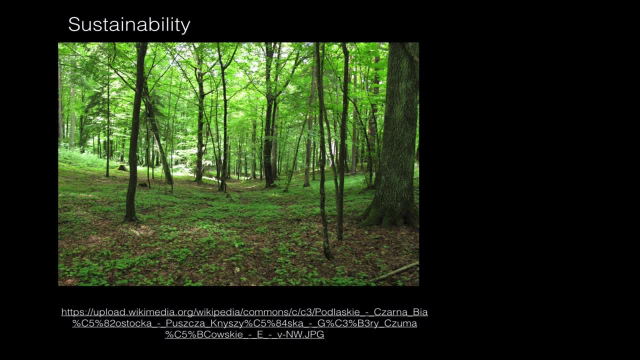 that it provides in order to give us a product. And by doing this, if I use it sustainably, that means that I'm allowing for the forest to regrow before I clear, cut it before I cut everything down. So it's not the idea. sustainability is not the idea that I can never take anything. 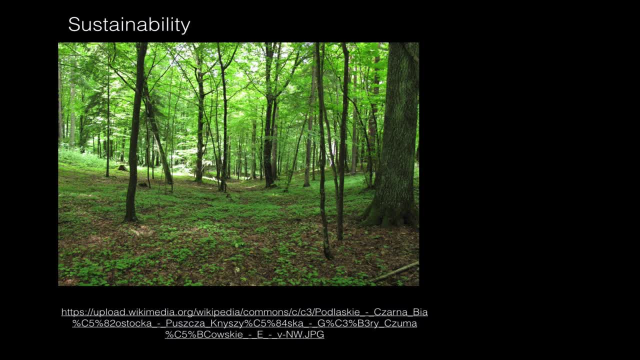 from the environment, But rather it's the idea that we are managing it so that it provides for future generations. So we're using the resources, but we're using them in a way that it allows them to regenerate and provides minimum harm to the environment. If I look at it on the reverse side, if I look at 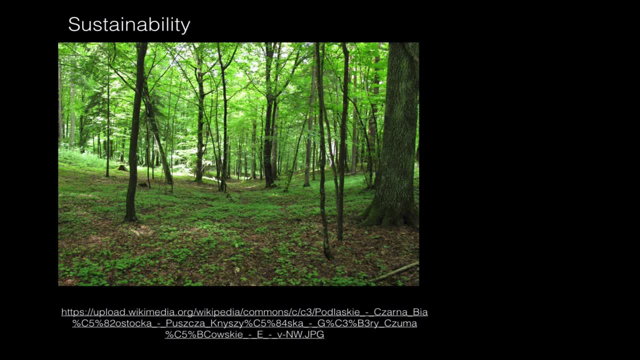 unsustainable practices. in that case, I would cut down the forest and I wouldn't allow it to regrow. So I'd take away more than what it can provide. So I'd take away more than what it can provide for me, And that moves into an unsustainable action. 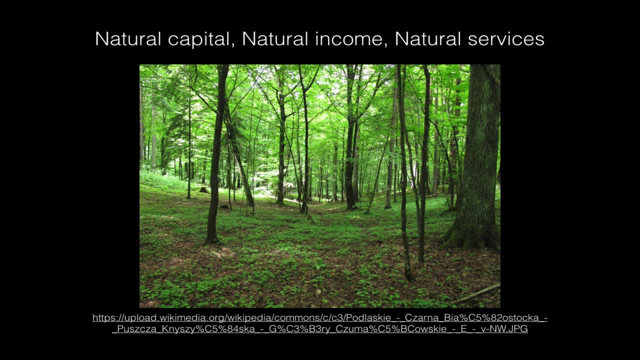 When we talk about sustainability, these three words- natural capital, natural income and natural services- often go hand in hand with them. So natural capital is a bard from a term that economists use, And when economists talk about capital, what they're talking about is the means. 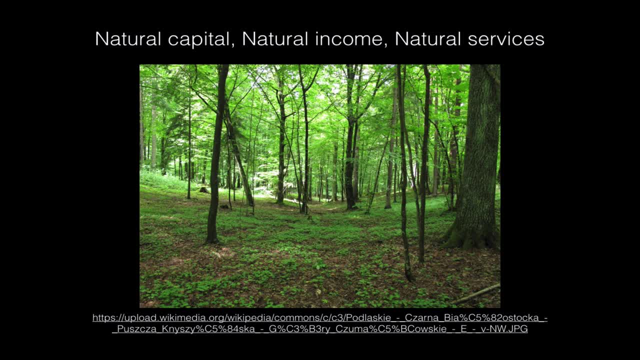 of production. So things like factories, tools or machines And these things are the means of production. These things, the factories, the capital, are used to create goods which provide income. So natural capital is a term that we use for natural resources that can provide a natural income of. 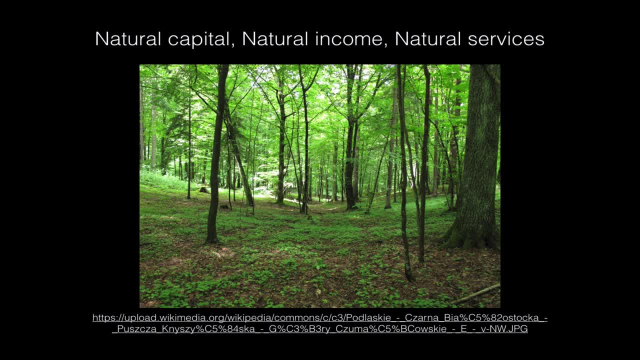 goods or services. So again, here's my forest. My forest itself is the natural capital. It provides a natural income in the form of timber and a natural service in the form of erosion, allowing for groundwater regeneration. So our natural services tend to be our processes. 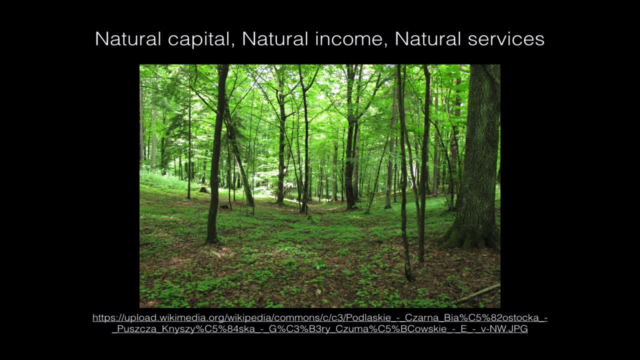 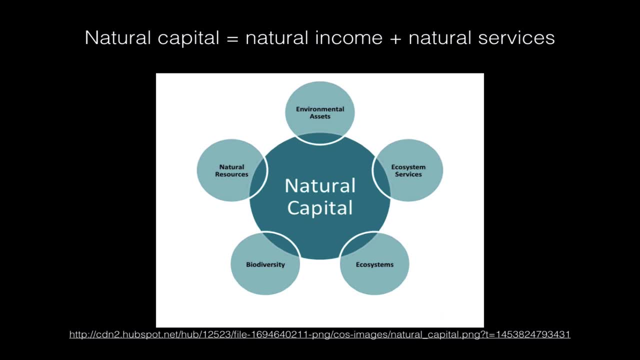 Our natural incomes are the goods that can be provided to us, And put those two things together and what we have is the natural capital. If I look at it in another way, here's this circle, And in the center of the circle I have natural capital, And all of these different parts make 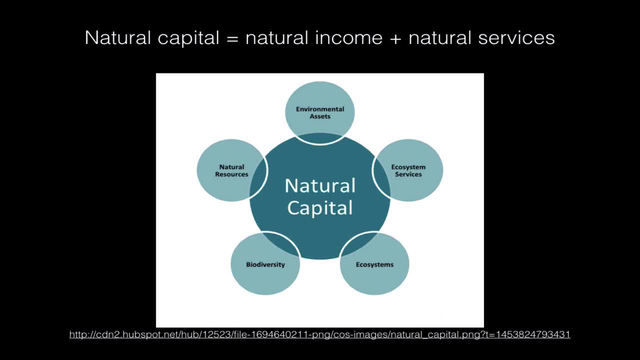 up my natural capital, So my natural resources- things like oil fit into this category- My assets. that goes back to the idea of that timber that we were just talking about. Ecosystem services, photosynthesis, the water cycle, the carbon cycle, the ecosystems. 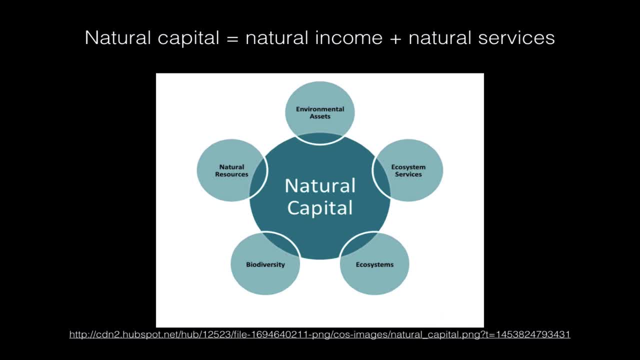 things that we talked about earlier, the tropical rainforest and all the things that they provide, such as giving the earth more, or the cleaning of the air, air purification, biodiversity, the range of organisms that we have on the earth- All of these things make up little bits of natural capital, And again, natural capital. 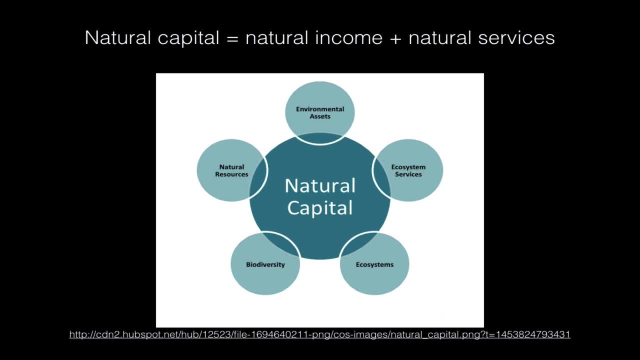 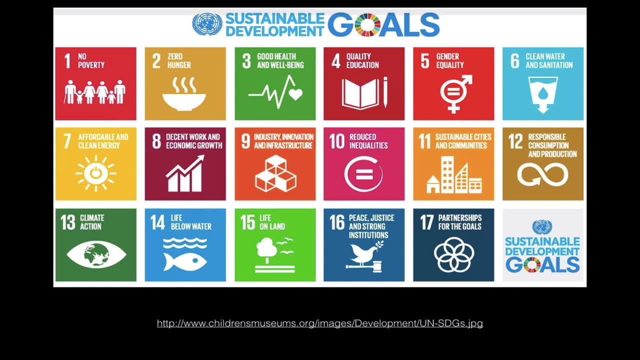 is made up of our natural income, the goods and the natural services, the processes that the environment can provide us. Sustainable development is an idea that says we can meet the needs of the present without compromising The ability of future generations to meet their own needs, And the idea was first popularized in. 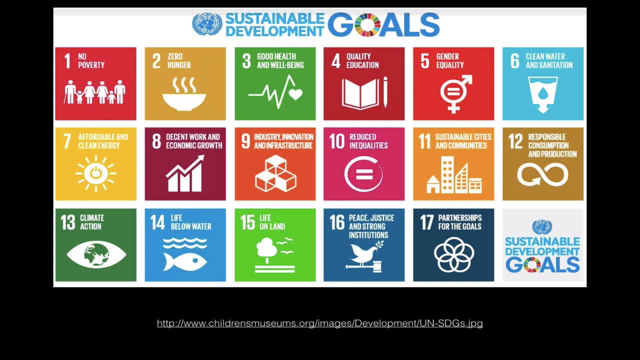 the late 1980s by the Brundtland Commission, which was a report to the United Nations and it was called Our Common Future. And Our Common Future focused on three main pillars: economic development, social development and environmental protection- And it called for a 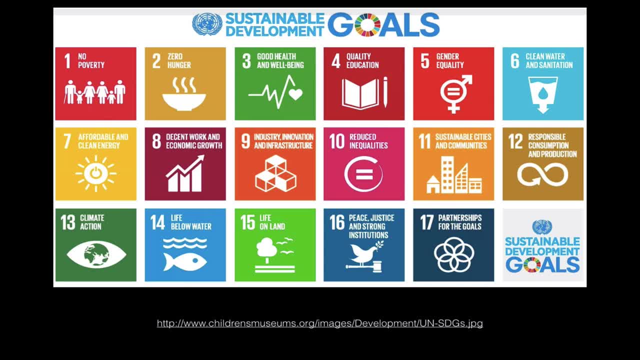 balance between those things. Over the past decades there's been a lot of talk about the economic development, social development and environmental protection, And they looked more at global poverty, health, environmental quality and social justice. So our latest thing from the 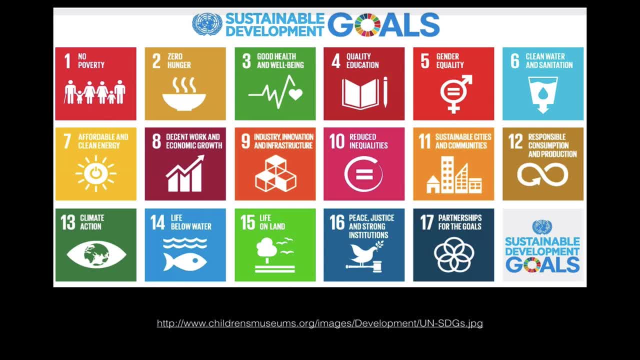 UN is our sustainable development goals, and these were implemented in January 2016.. So, starting in January 2016,, UN member nations are expected to begin enacting policies and legislations to help meet these goals. And these are the 17 goals that are needed for sustainable development. 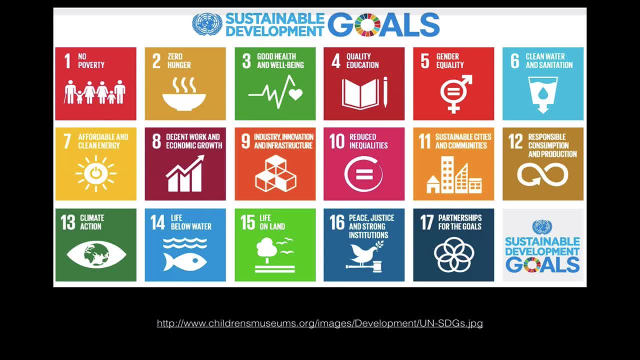 So some of these goals include protecting air, land, water, natural environments, and there's lots of talk about the ocean as well, because we're realizing that our ocean has a lot to do with ending things like hunger, giving us energy and relying on climate change. So there's a lot of 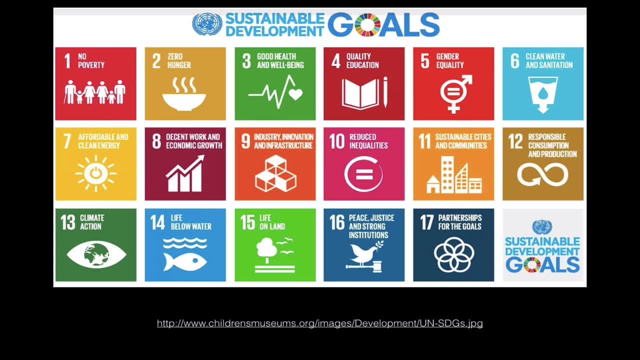 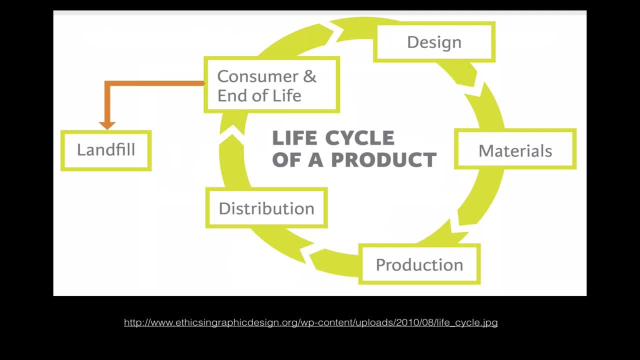 things that go into here On the environmental side and on the economic and social side as well. So let's think about this idea of sustainability again. And sustainability is using global resources at a rate that allows the natural regeneration and minimizes damage to the environment. So, again, 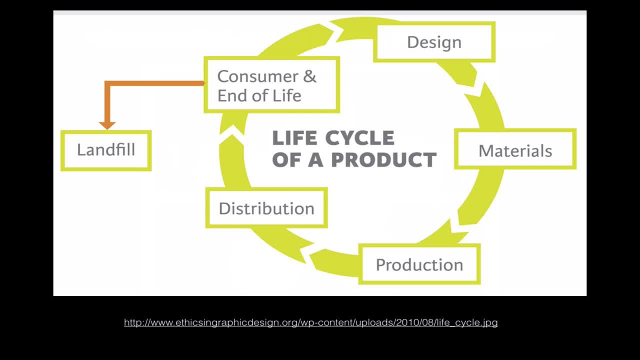 it's smart use, and this means that we use our resources wisely. and one idea that we talk about more frequently when we're discussing sustainability is the idea of goals. It's not just the goals that we're discussing, it's really just the goals that we're starting to use for ourselves, because we're 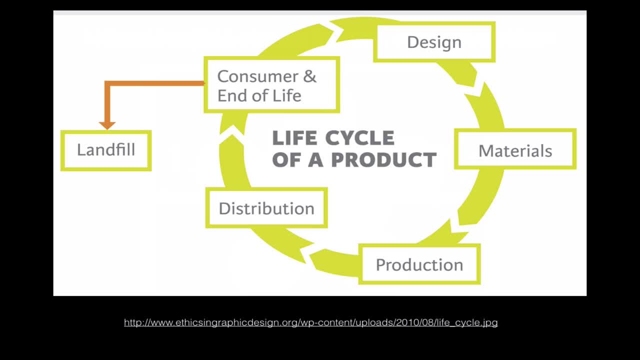 always looking at the goals of those goals, And so, for me, that's what I'm starting to see as a to think about, and is this idea of a life cycle. When we create something, we want to design it in a way that 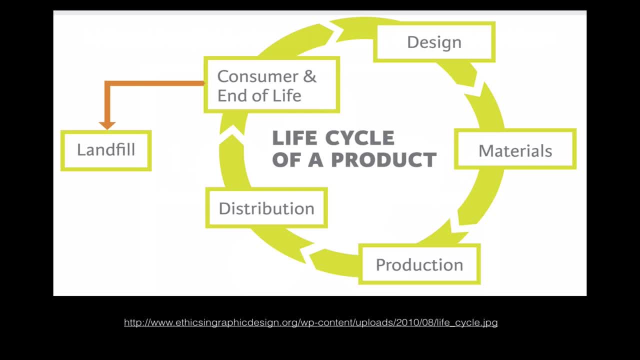 it lasts longer, that we use less materials, that we use less resources during the production and the distribution of the product. We want to keep our product in use as much as possible before it ends up in the landfill, So what we used to call this was the idea of cradle to grave. 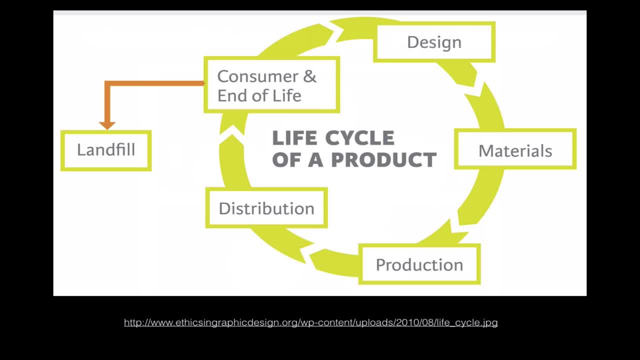 that we needed to take in consideration our environmental impact, not only in the production of our materials and our things that we use, but also in the creation, the delivering and the eventual disuse and the discarding of it. And this kind of moves us, helps move us into the 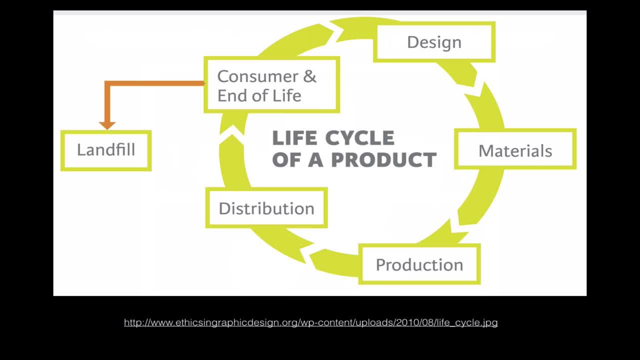 direction of a sustainable development idea. If we're considering more than just the creation and the end of it, if we start thinking about the whole process involved with our life cycle, then we start to think in a more sustainable way, because we're thinking of everything that's involved with making a product. This is a good time to briefly talk. 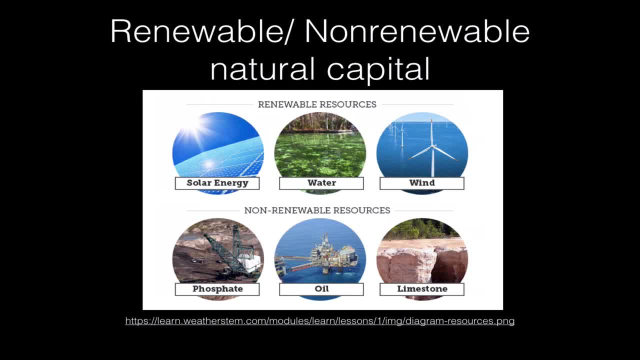 about renewable and non-renewable natural capital Again. natural capital is another word that we use for natural resources, And this is something that goes that we talk about a lot more in depth later on in the syllabus, but I just want to briefly mention our two main ideas of.